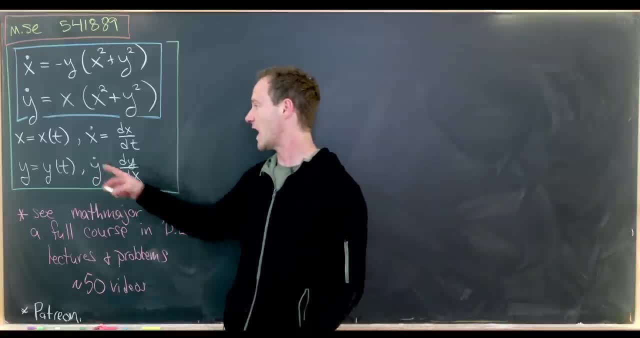 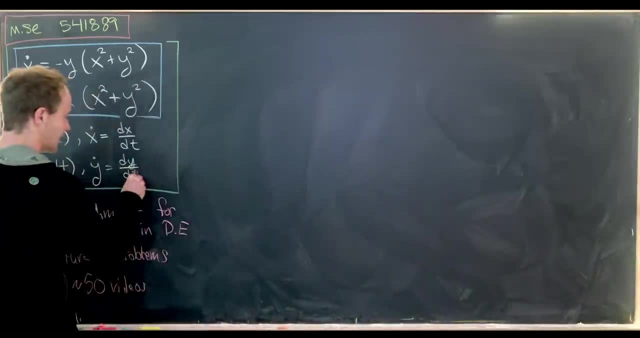 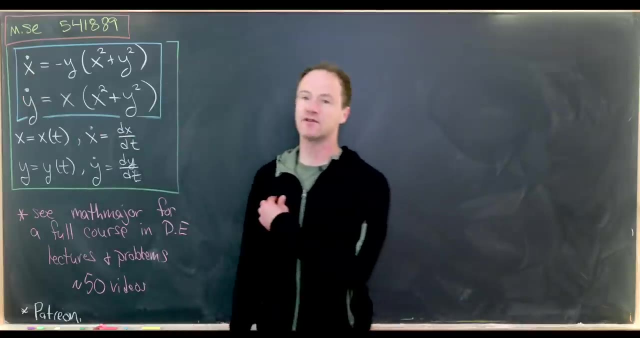 is equal to the derivative of x with respect to t and y dot is likewise the derivative of y with respect to t. that should be. Who put a comment there before I fixed it? Okay, so the system of differential equations is: x dot equals negative y times x squared plus y. 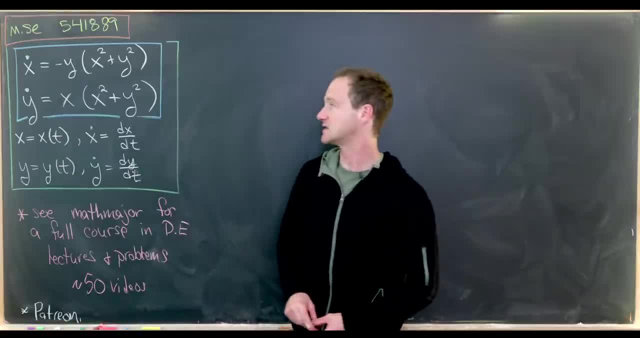 squared And y dot equals x times x squared plus y squared. And anytime you have a nonlinear differential equation, let alone a system of nonlinear differential equations, you know that there's probably a difference between x and y. And if you have a nonlinear differential equation, 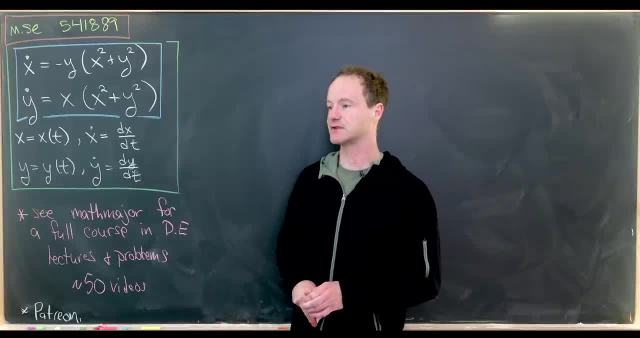 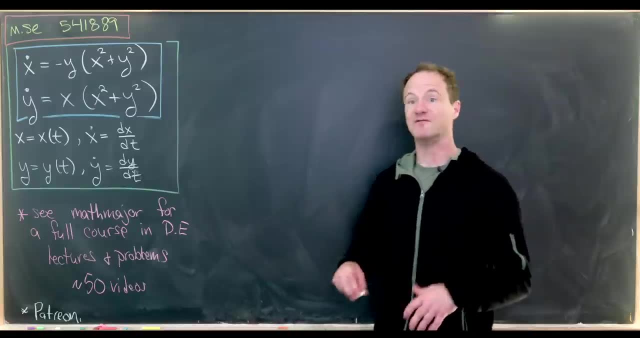 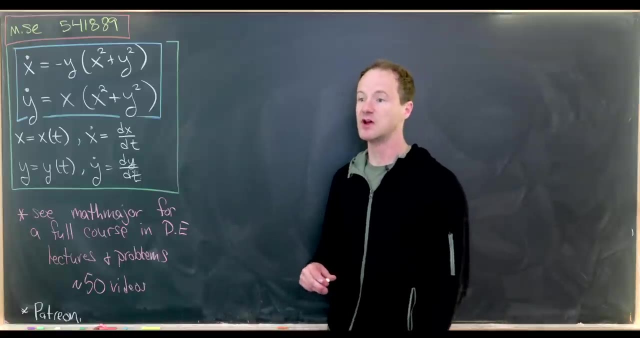 that's going to be a trick that will allow us to come up with a fairly simple solution, And that's because the general theory of systems of nonlinear differential equations is a very difficult general theory And it's very easy to write down these types of differential equations that have no 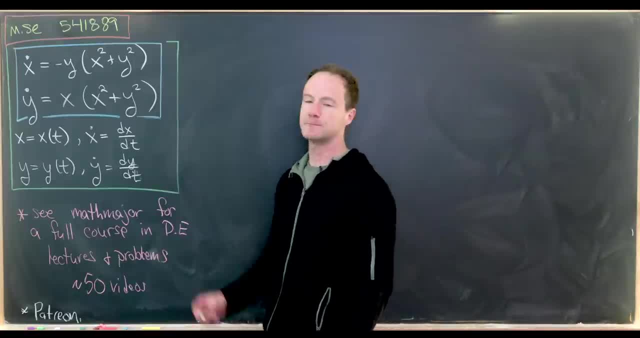 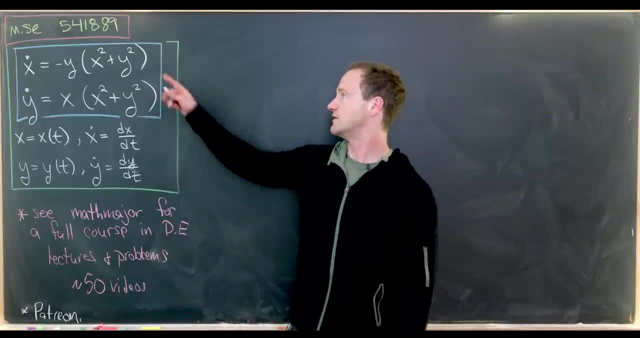 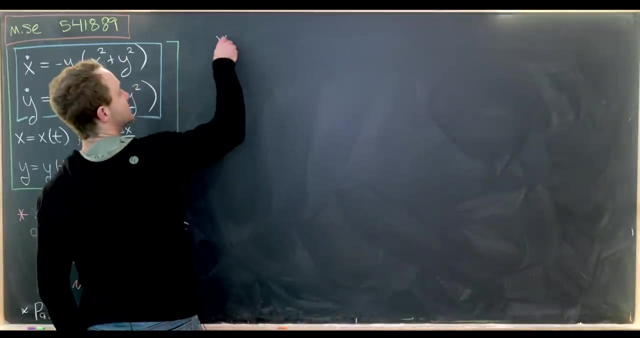 simple solution. Okay, so what's the trick here? I think our big motivation is that we've got x squared plus y squared in both of these terms, And that's because we have a nonlinear differential equation, And that motivates me to make a change of variables into polar coordinates. So let's do. 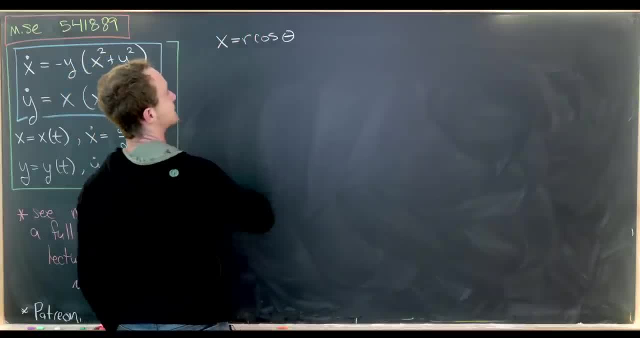 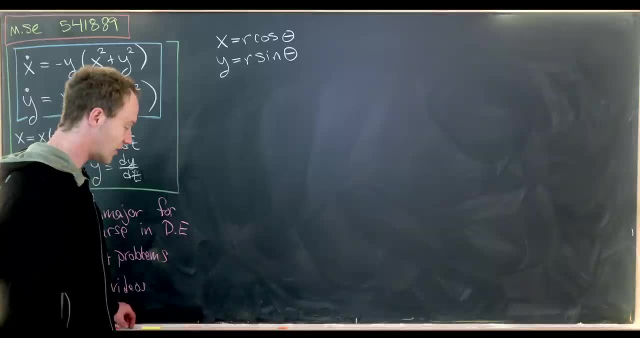 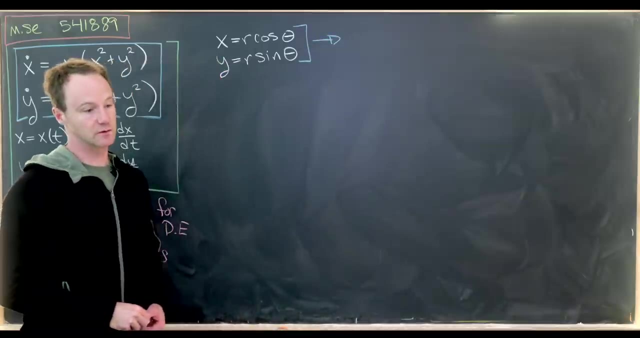 that We'll set x equal to r times cosine theta And we'll set y equal to r times sine theta. And although we won't use this explicitly, it's a nice exercise in the product rule and the chain rule to find the derivative of the x with respect to t and the derivative of y with respect to t in. 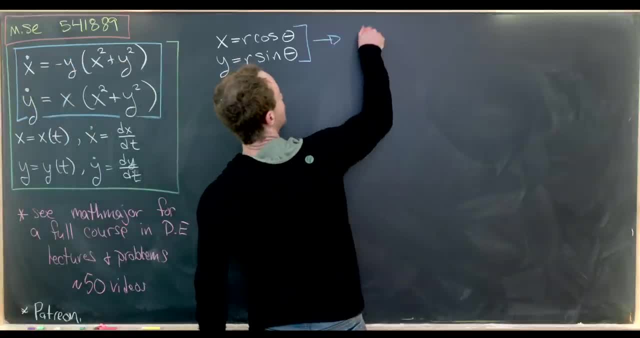 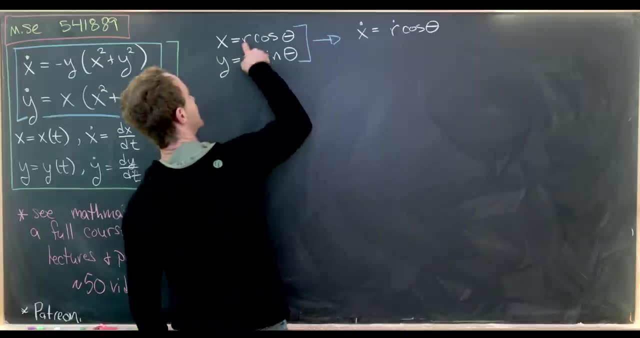 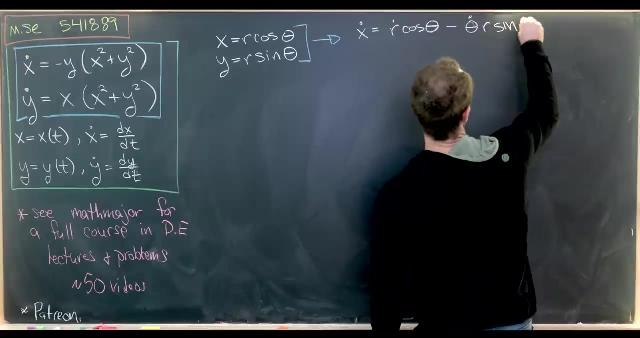 terms of these new polar functions. And in fact what we have is x dot is equal to r dot times cosine theta. So that's taking the derivative of r And then we'll have minus theta dot times r, times sine theta. So notice, I had to use the chain rule there. I took the derivative of cosine and it. 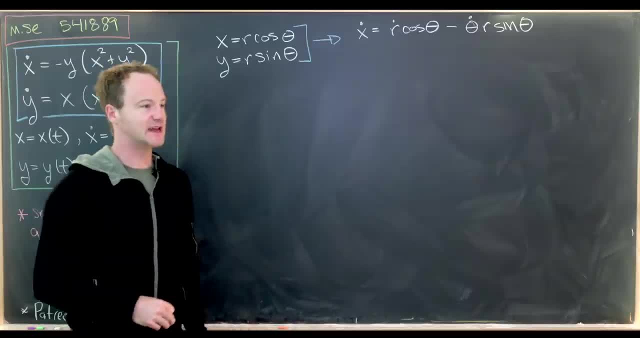 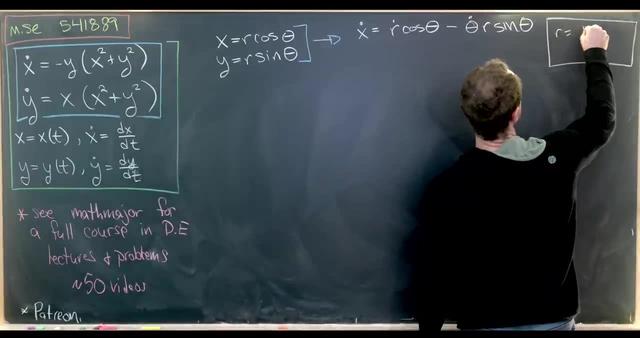 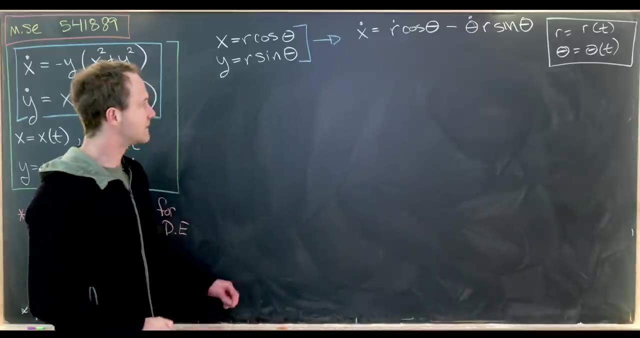 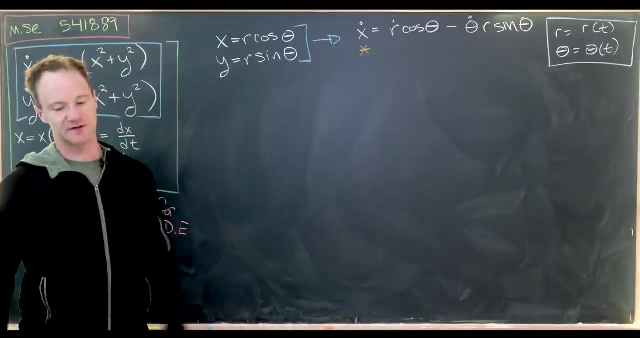 became negative sine. Then I had to take the derivative of the inside function, Because with this setup it's important to realize that r is a function of t and theta is also a function of t. Okay, so maybe as a little exercise, you guys should write down what y dot is in terms of this. 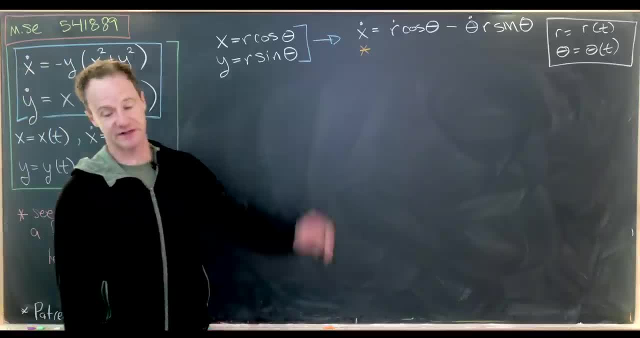 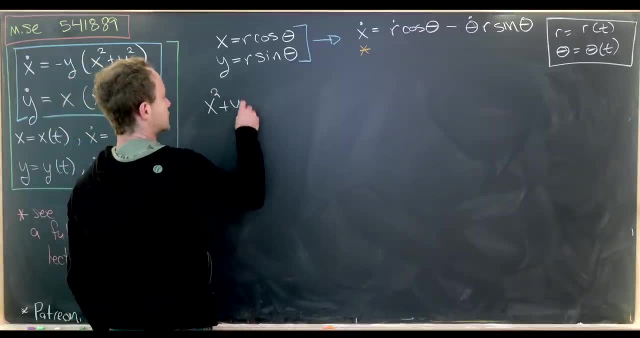 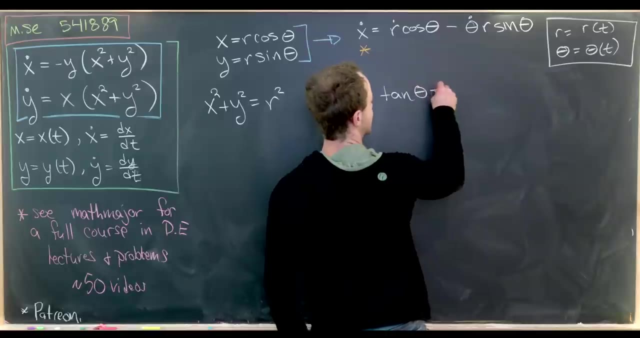 sort of expansion. Like I said, our trick will not rely on explicitly writing that out. Instead, what we will use is the fact that x squared plus y squared is equal to r squared, And the fact that the tangent of theta is equal to y over x, And so 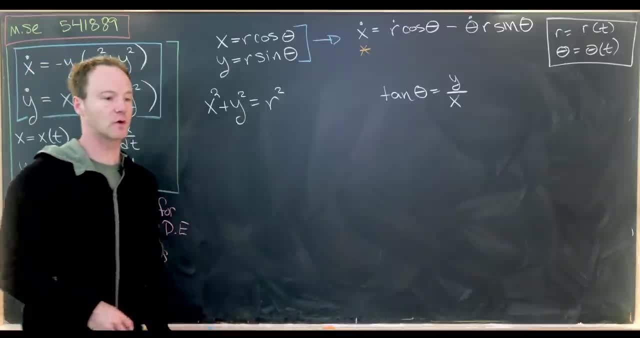 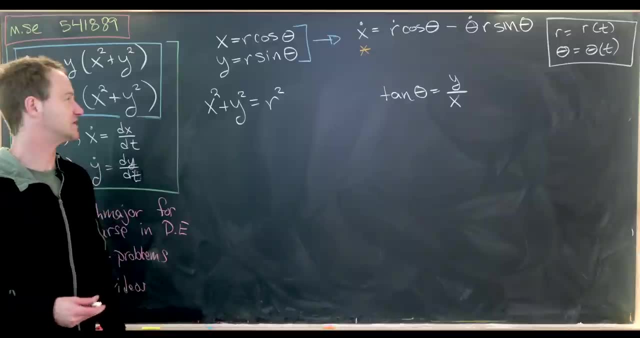 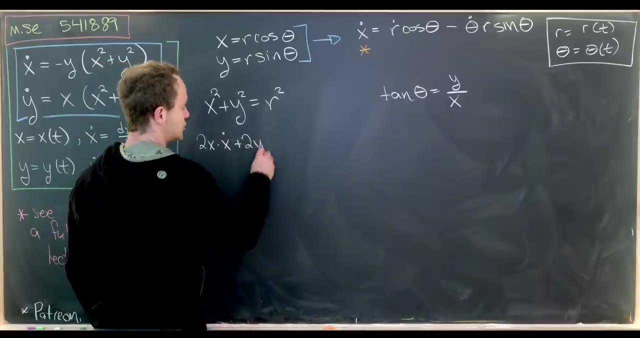 that's just standard rules for converting polar coordinates to rectangular coordinates and back again. And now we can take derivatives of these equations, thinking about implicit derivative rules. Okay, so this is going to give us 2x times x dot plus 2y times y dot. 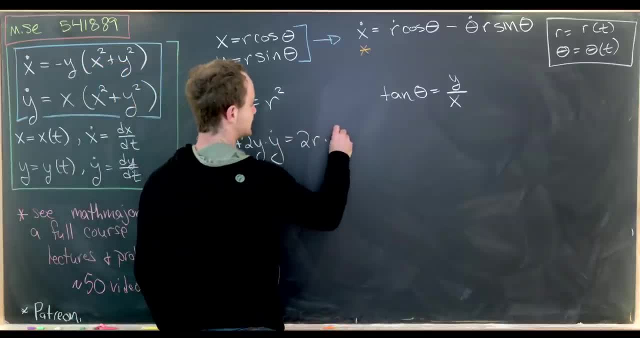 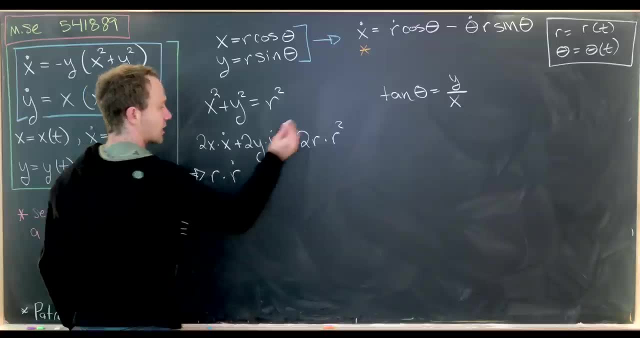 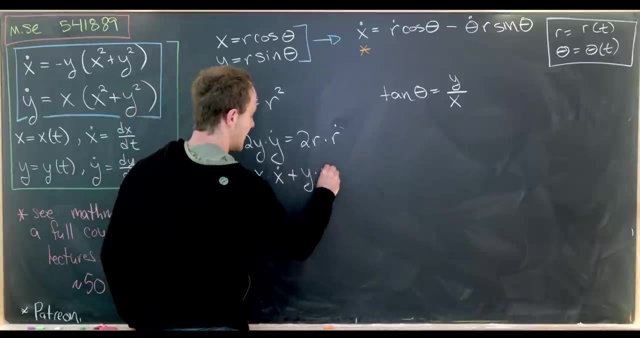 Using the chain rule, equals 2r times r dot. Now clearly we can divide by two. that'll give us r times r dot is equal to x times x dot plus y times y dot. But check it out: y dot and x. 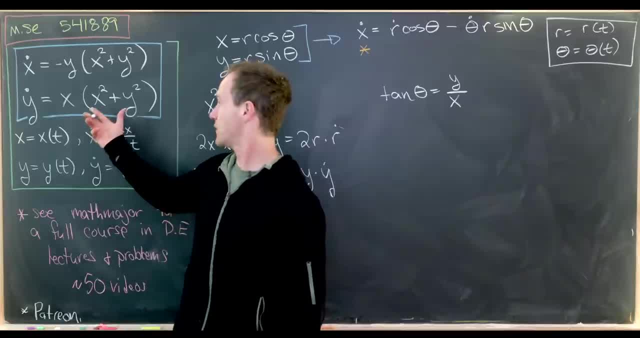 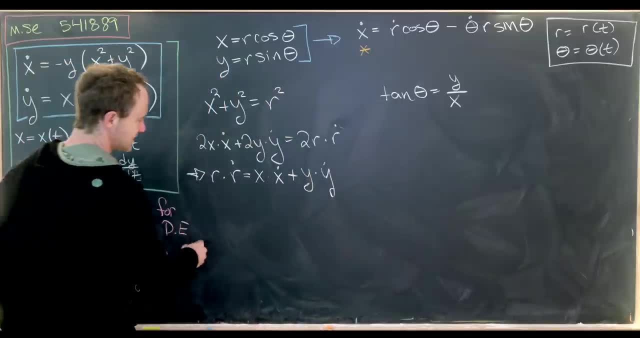 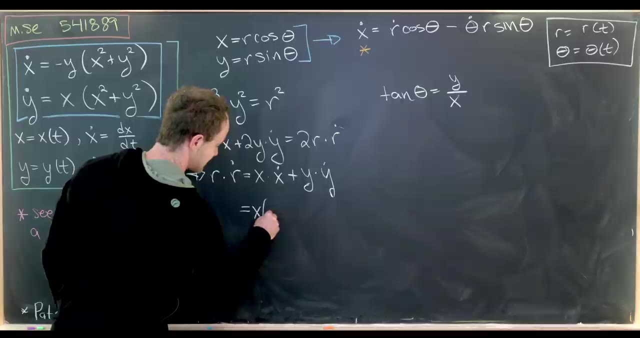 dot are suspiciously similar. They both have this x squared plus y squared. this one is attached to a and y dot is attached to an x. So let's see if that provides us any simplification. So we'll have x times x dot, but x dot is negative. y times x squared plus y squared, but that's negative y. 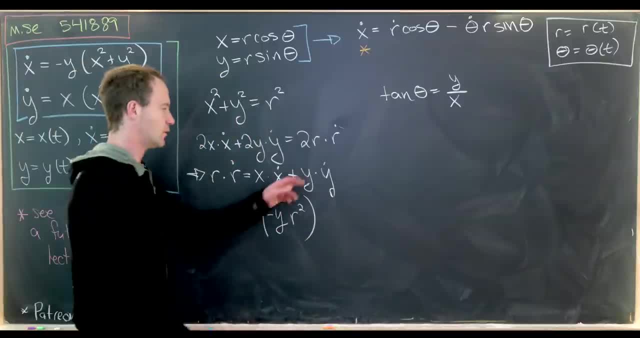 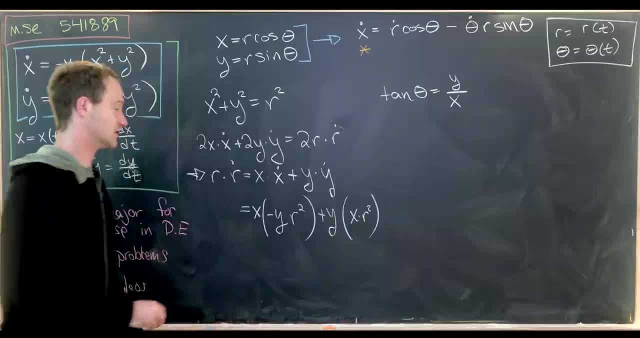 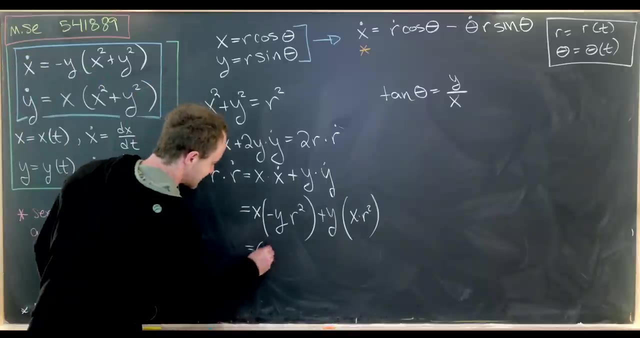 times r squared, Then y times. y dot will give us y times and then this will be x times r squared, similarly. But look at this: This is negative: x- y r squared and this is positive: x- y r squared. So that's going to cancel down to zero. So what does that tell us? We have r times. r dot is equal. 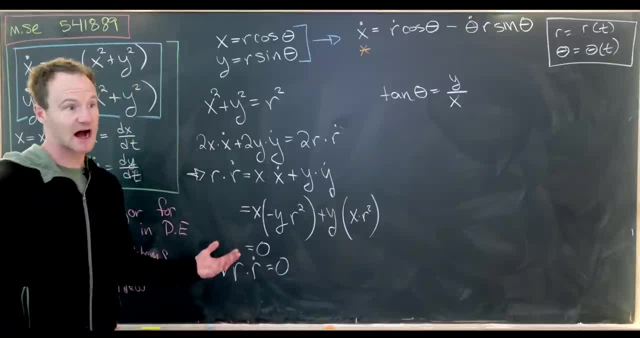 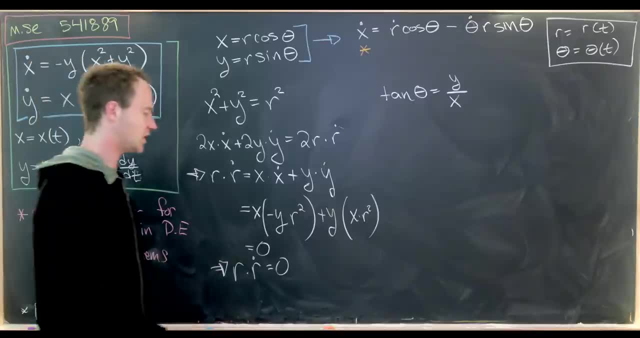 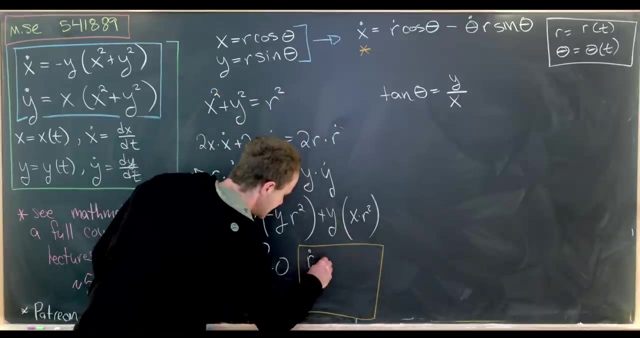 to zero. So that splits into two cases: Either r is equal to zero or r dot is equal to zero. But notice that if r is equal to zero, then r dot is also equal to zero. So any way you put this, we get that r dot is equal to zero, But if r dot is equal to zero, that's what kind of function has. 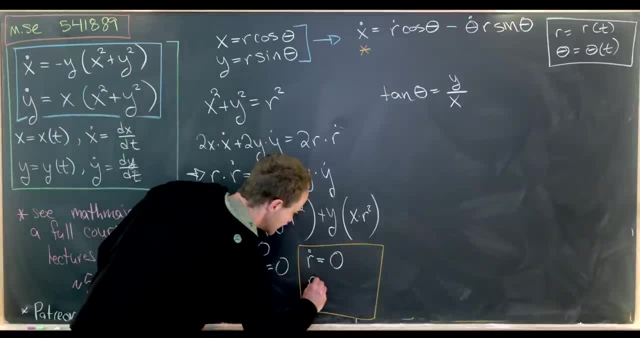 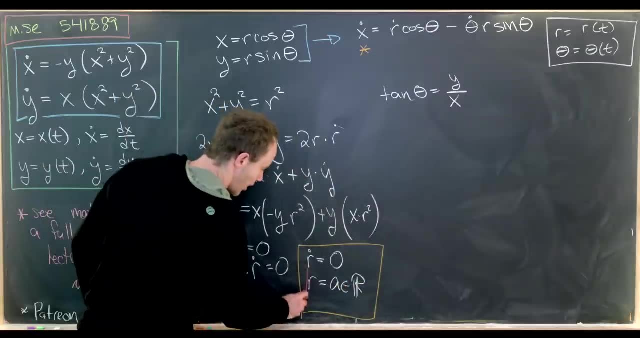 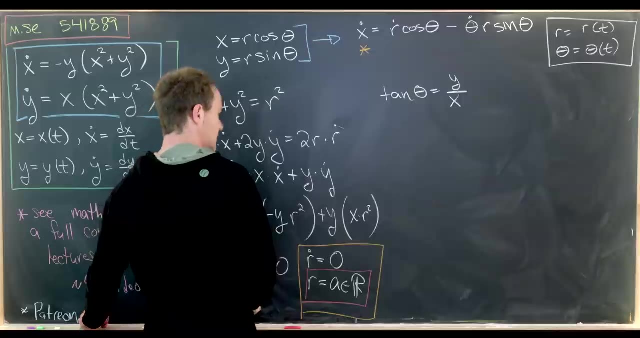 the derivative. that is zero and that's just a constant function. So we have: r is a constant. I'll call this constant, maybe a. So there we know what r is. It is just this constant a. So that's good news. Now we're going to play a similar game over here, with this tangent. 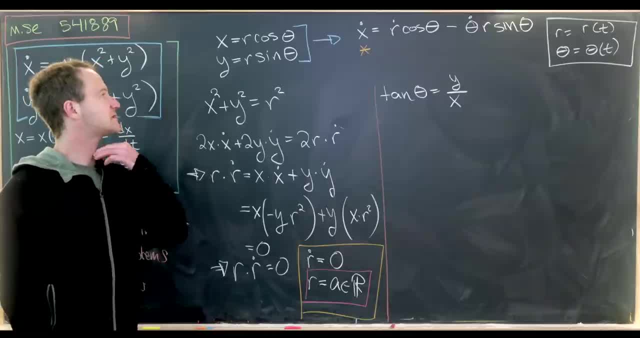 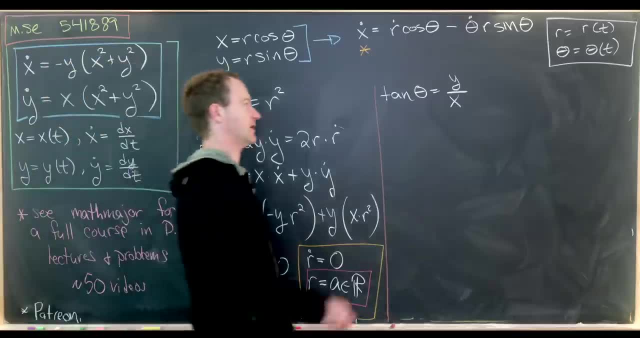 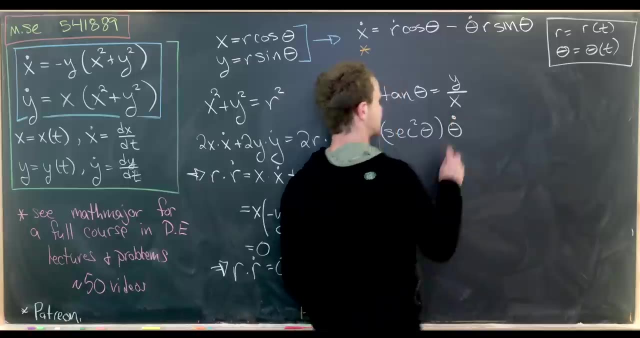 theta equals y over x. Again, we get that just because sine over cosine is equal to tangent. Okay, so let's take the derivative of both sides. So the left hand side will give us secant squared of theta times theta dot. So that's using the chain rule. And now over there on the right hand. 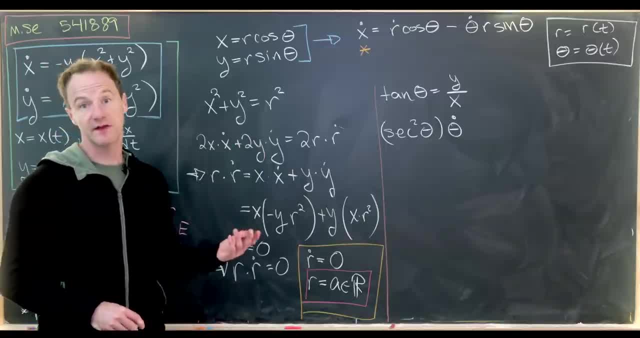 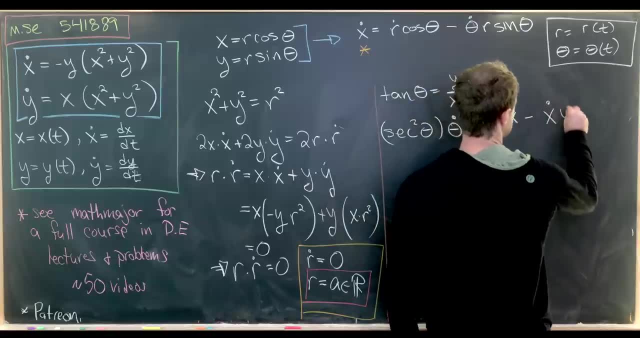 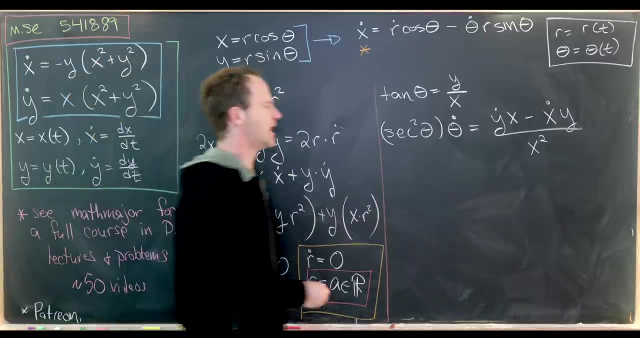 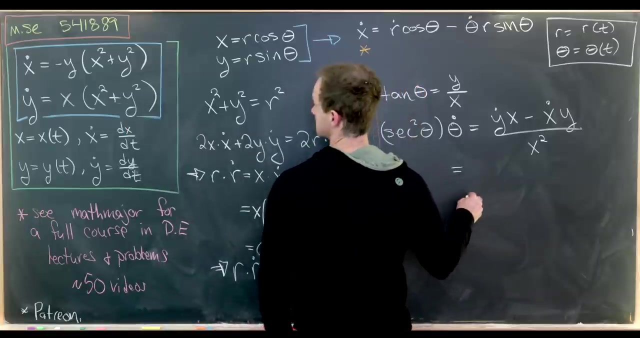 side. we'd probably like to use something like the quotient rule, So that will give us y dot times x minus x dot times y over x squared. Okay, nice, But now we know y dot and x dot from this situation up here. So that's going to give us, let's see, x squared times r squared. But notice: 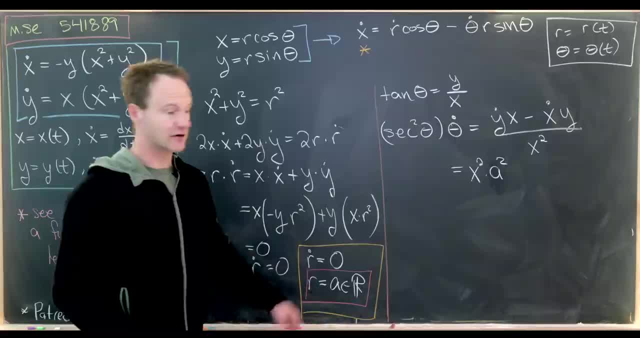 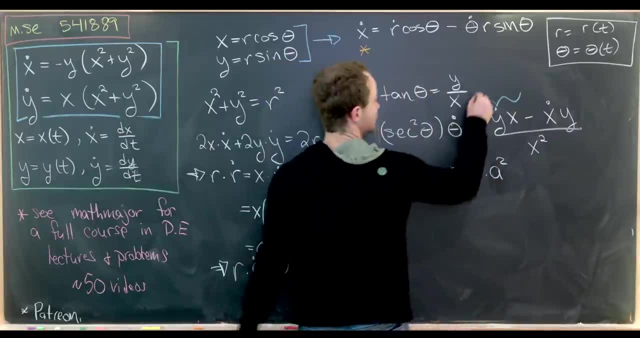 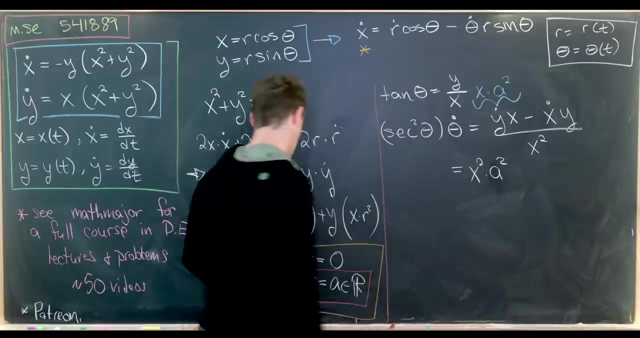 r squared is just a squared. So just to reiterate what happened there, I took this y dot and I'm going to expanded it into x times x squared plus y squared. but x squared plus y squared is R squared. but R is this constant a from our previous work and now we'll do. 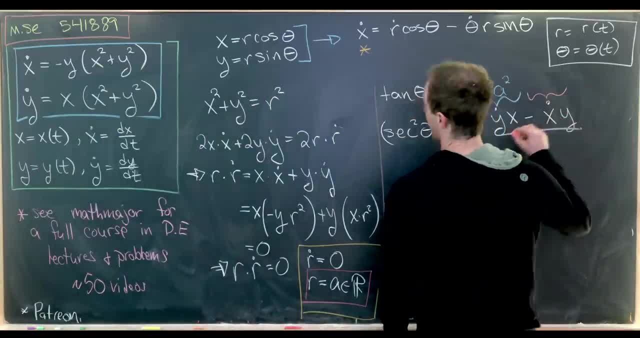 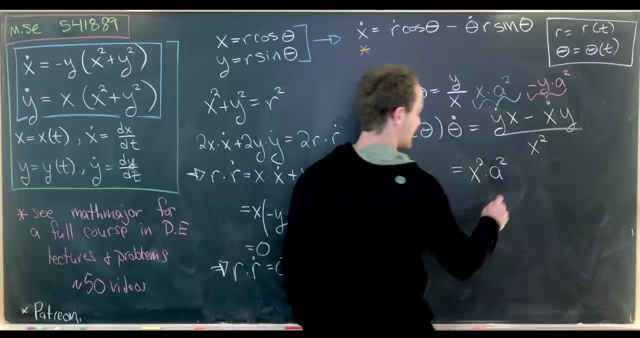 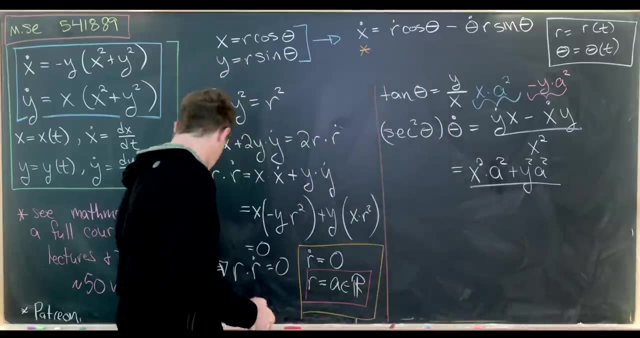 a similar expansion over here. we know x dot is equal to negative y times a squared for the same sort of reason. so let's notice, those minus signs cancel and we get plus y squared times a squared. and now let's notice that this is all over x squared. but before we put x squared there, let's maybe do a little. 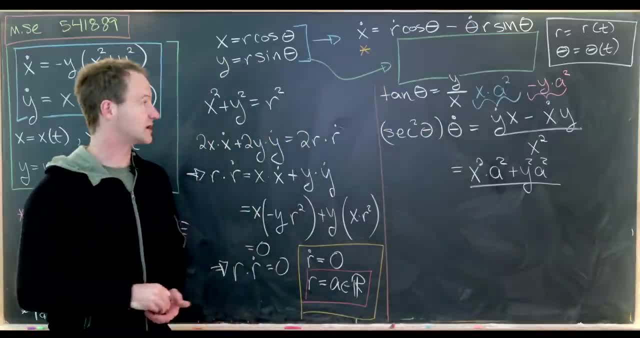 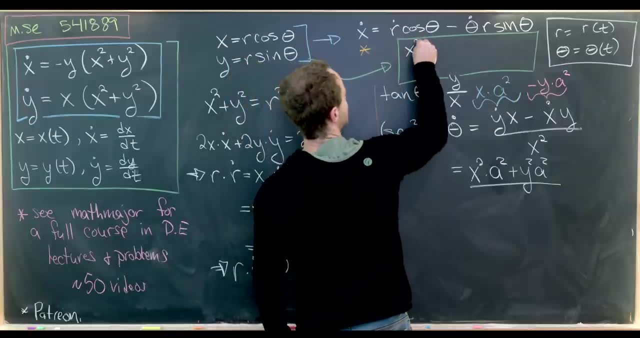 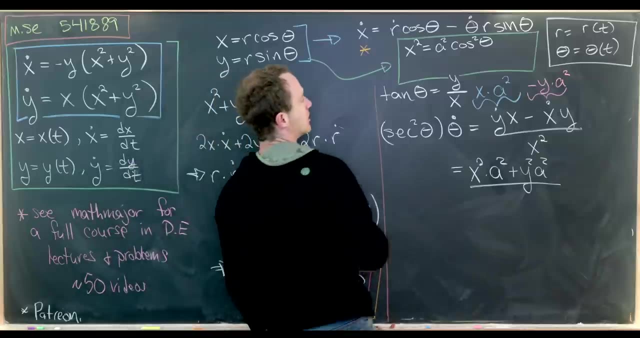 bit of a calculation which will allow us to maybe streamline this process. okay, so let's notice that x is R cosine theta. that means x squared is R squared, which is a squared cosine squared theta. so that means we're going to get plus y squared times a squared. and now let's notice: